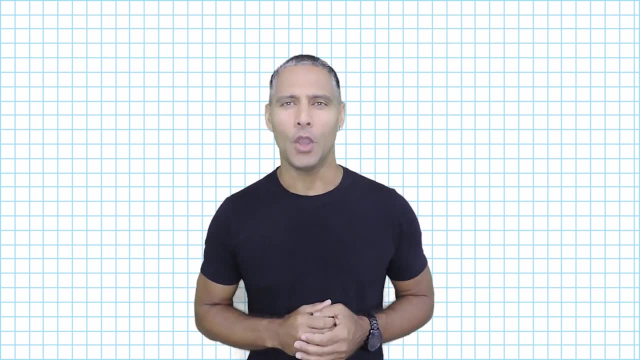 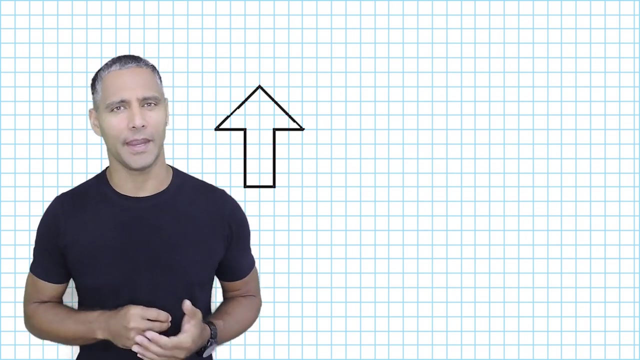 We are not going to graph any transformations in this video. We are simply just going to work on recognizing and categorizing the different kinds of transformations. The word transformation simply means that something is undergoing a change. Let's start by changing or transforming the arrow shown on the screen. 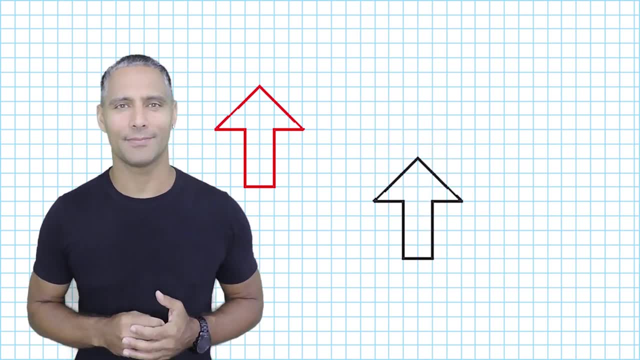 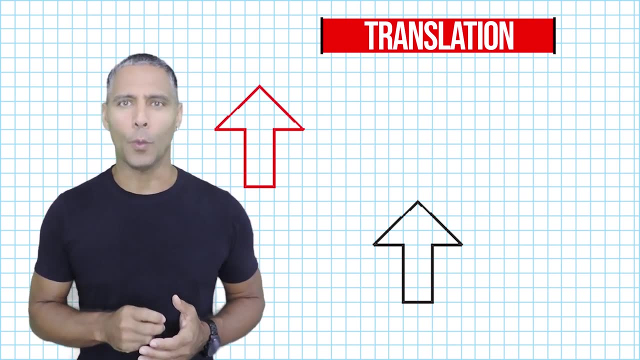 The type of transformation shown is called a translation. For a transformation to be identified as a translation, here is what must be true: The shape must be oriented in the same direction after it is moved. Notice that the arrow on the screen remained pointed upwards after it was translated. 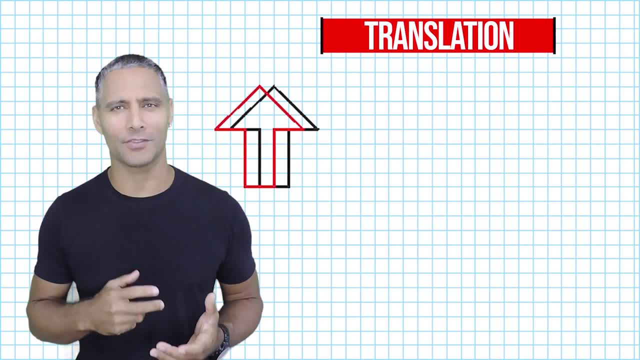 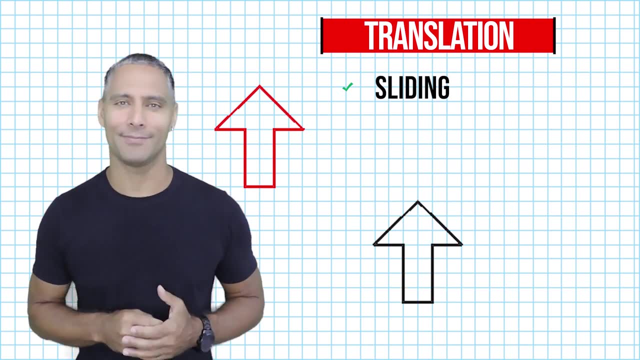 Also notice how it appeared as if we were sliding the arrow across the screen. If it looks like an object is sliding, we can quickly recognize that we are dealing with a translation. Also, notice that the object maintains the same direction as the arrow. The object is in the same shape and the same size. 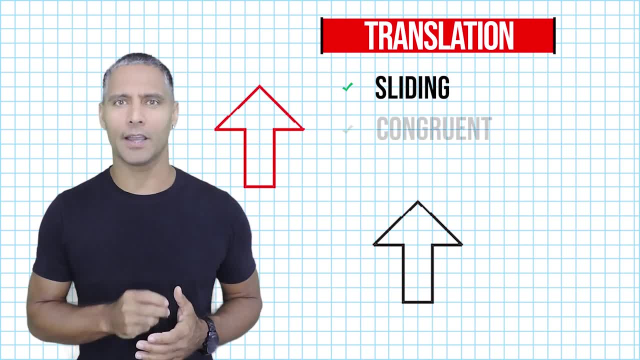 Anytime we translate an object, the resulting object will be congruent to its original. Because translations result in objects being congruent to their original, we must categorize any translation as a rigid transformation. A rigid transformation is any type of transformation that did not change its shape or its size. 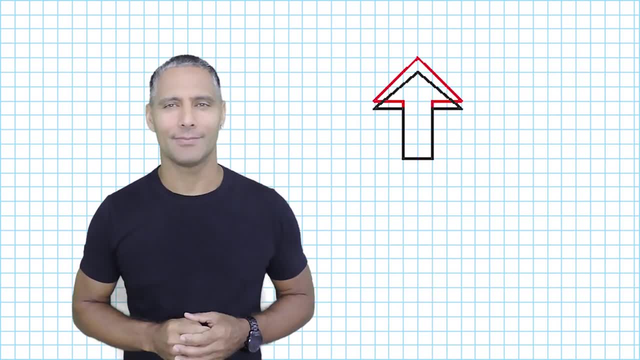 All right, let's take a look at another type of translation. Notice that the arrow in this case is not pointed in the same direction, so we know that it is not a translation like the first example. This type of transformation is called a reflection. 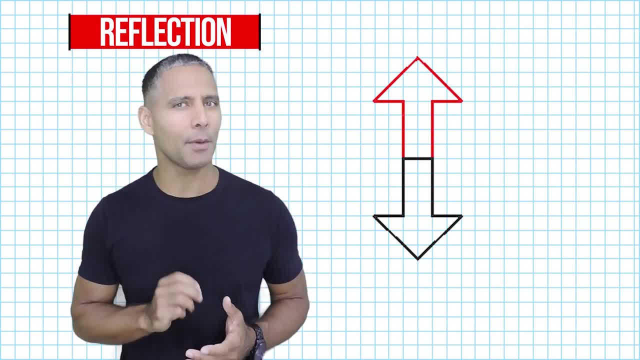 A reflection will appear as if the original image was flipped over some imaginary line. The line that it appears to be flipped over is called a line of reflection. A reflected object should always be the same distance away from the line of reflection as the original object. 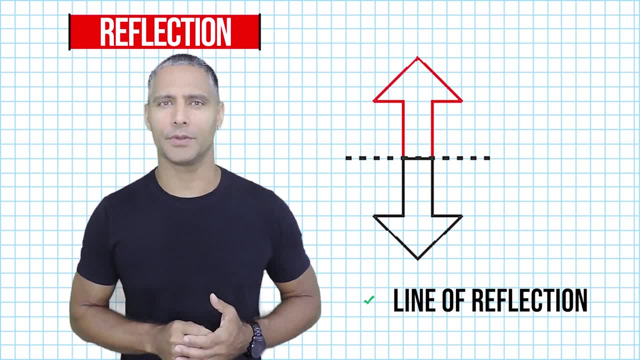 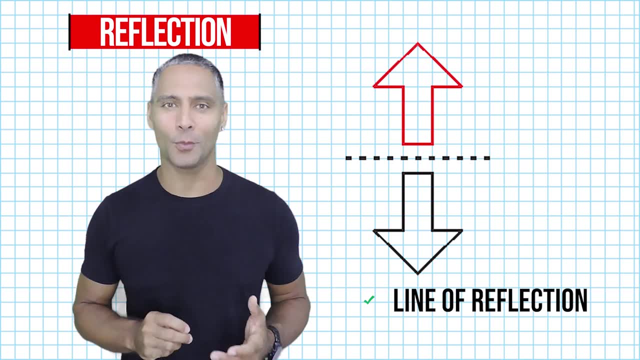 Notice that the original image was flipped over some imaginary line. Notice how both arrows are currently touching the line of reflection. If we move one arrow, one unit, away from the line, we must move the other arrow one unit away from the line as well. 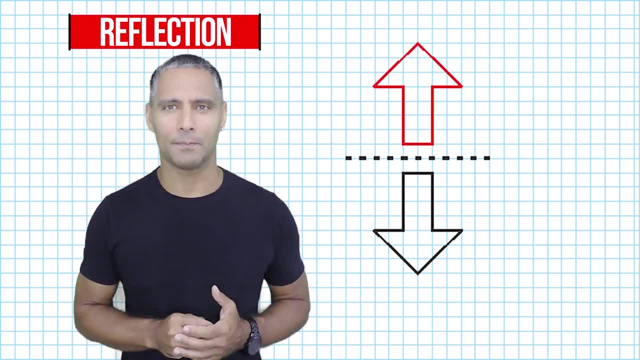 Think about the line of reflection like a fold in a piece of paper. If you were to fold the paper along the line of reflection, the two objects should line up perfectly. That is one way you can determine where a line of reflection would be located between two objects. 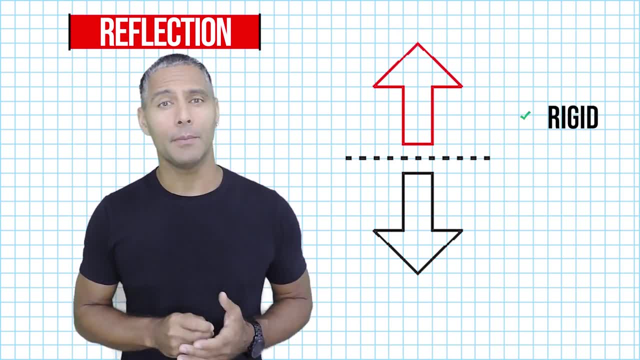 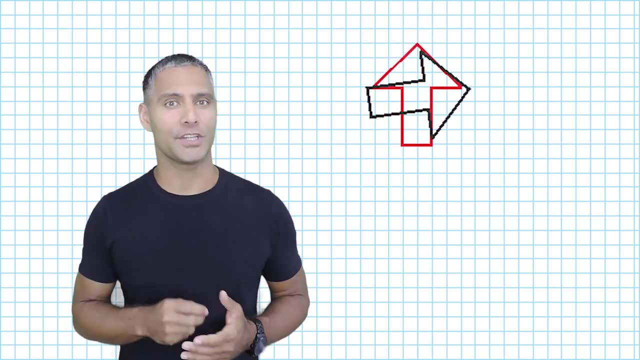 A reflection is an example of a rigid transformation. A reflection is an example of a rigid transformation because the result is congruent to its original. Now let's take a look at a third rigid transformation. This one is easy for most people to recognize. 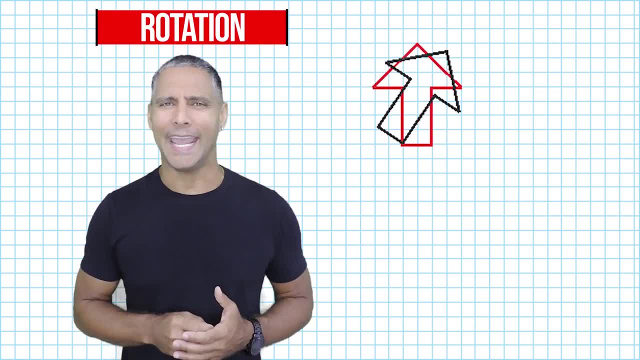 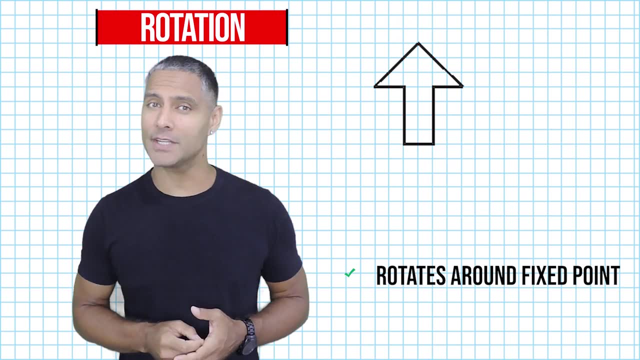 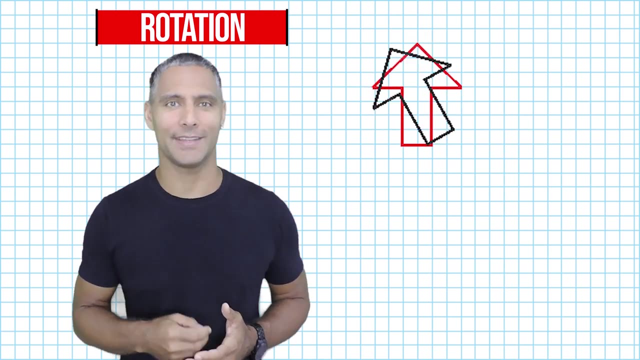 This rigid transformation is called a rotation. Any object being rotated will always do so around some fixed point. Sometimes that fixed point is located inside the object, like the example shown on the screen, and other times an object is rotated around a fixed point located outside of the object. 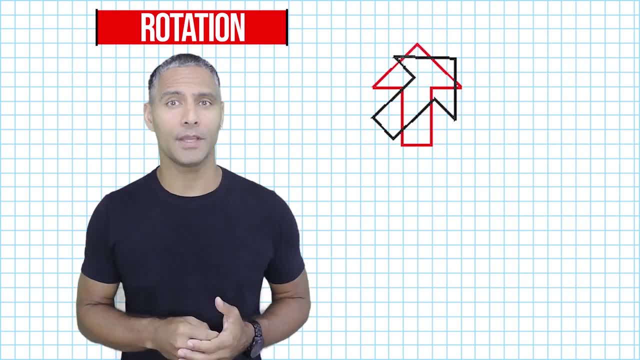 The fixed point may be the origin of a coordinate plane where the x and the y-axis intersect, or it may be any arbitrary point on the coordinate plane. Rotations may also be described by the direction that they are being rotated, whether it be clockwise or counterclockwise. 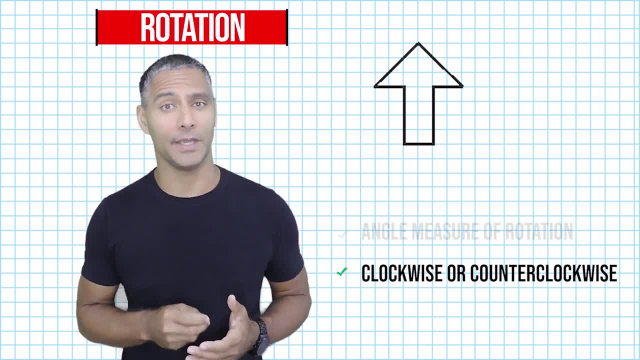 We also use angle measure to describe how far an object is being rotated. Now, remember this is just an introduction to transformations. We will get into specific examples in other video lessons. Now let's take a look at an example of a non-rigid transformation. 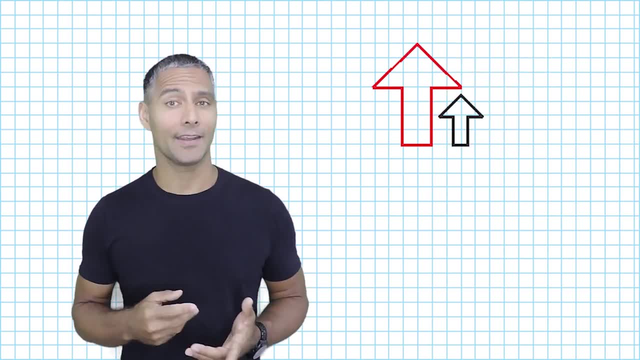 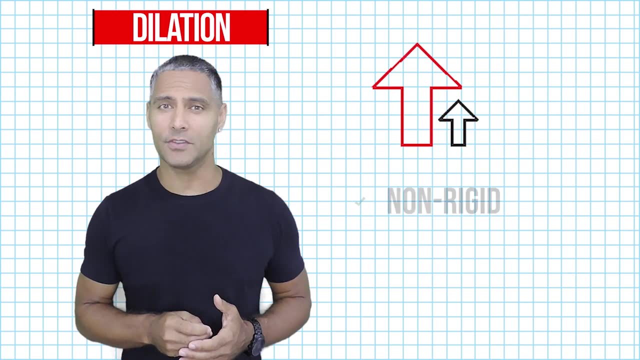 If you look at the arrow on the screen, we can see that it is shrinking and expanding. This kind of transformation is called a dilation. Dilations are non-rigid transformations because the size changes. Therefore, the two objects are not congruent to each other. 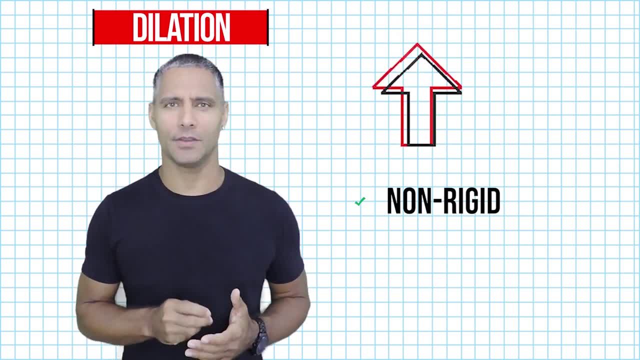 Although the sizes are different, we should notice that the shape is still the same. In fact, dilated objects will always be similar to their origin. Now remember, similarity is a mathematical concept which just means that objects are proportional to each other. 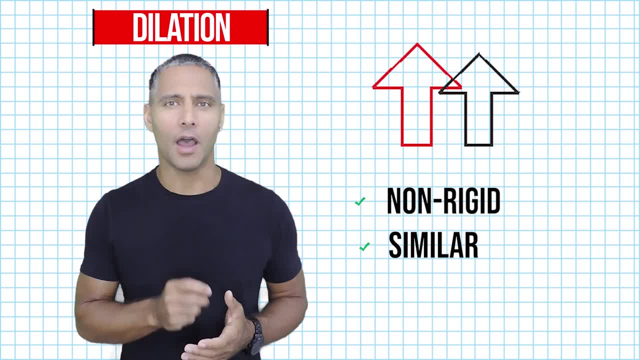 So if one side of our object became one half as large, all other sides of that object must be scaled down by a factor of one half. If one side became three times as large, all other sides must be three times as large or scaled up by a factor of three. 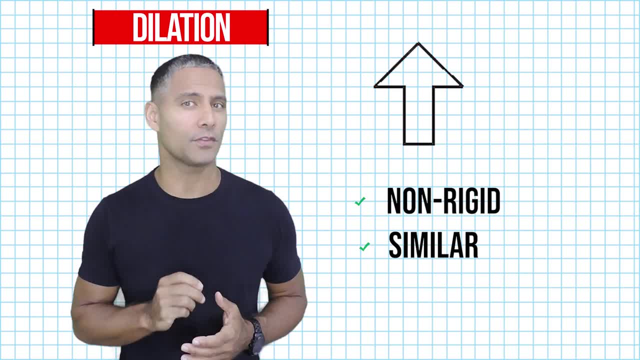 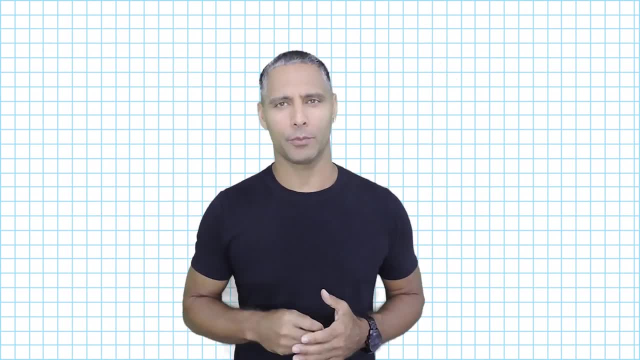 The dilation of an object can be performed in reference to a fixed point, which I examine in my dilation videos found on my YouTube channel. Alright, let's do a quick review. When an object is being slid around but remains pointed in the same direction, it is called a translation.